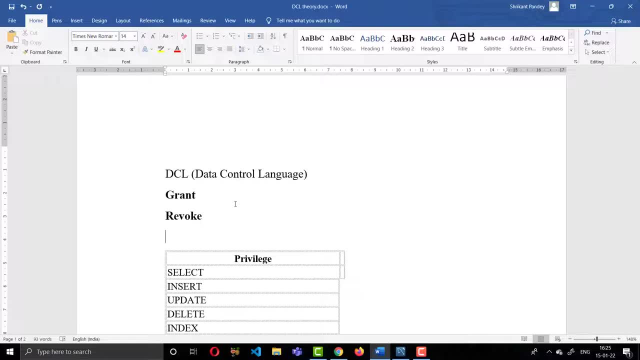 the some particular kind kind for user is applied. So let's understand what is the grant? So Grant is a grant command used to set the privilege to the user to the select or insert data, update the data and delete the data for the particular user. 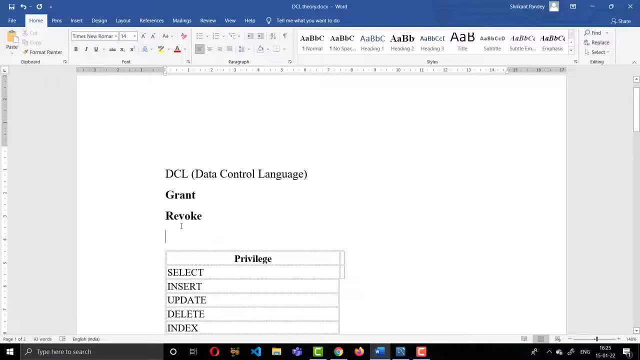 regular user in the table and revoke is used to suppose you have given the permission for the rom user. i want to take off this all the permission you have set for rom. so you do not give the permission for rom in that for the table. so for that purpose is use a revoke. 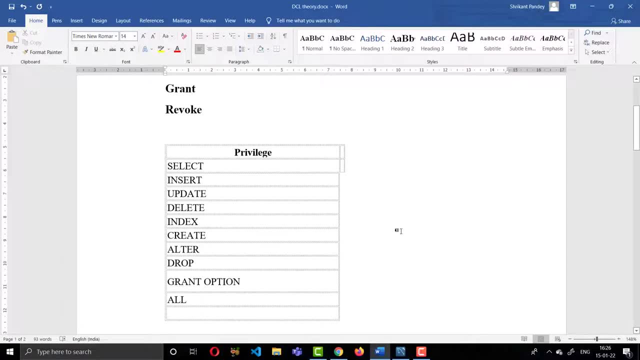 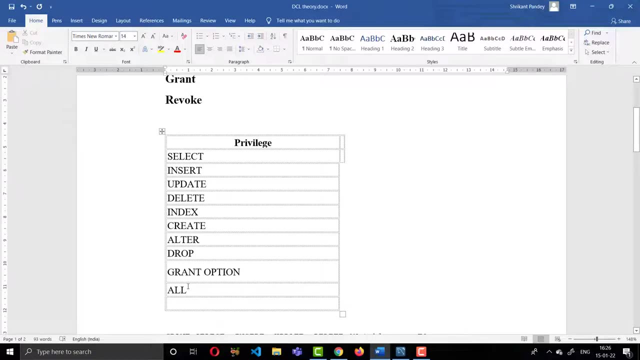 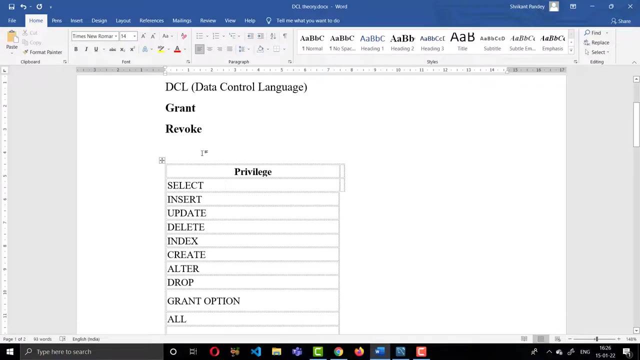 command. so there is some privileges are available, like select, insert, update, delete, index, create, alter, drop and grout option. this is all so you can, all the operation you can perform whatever you mention here. so now we understood. so let's i give the real example. suppose you 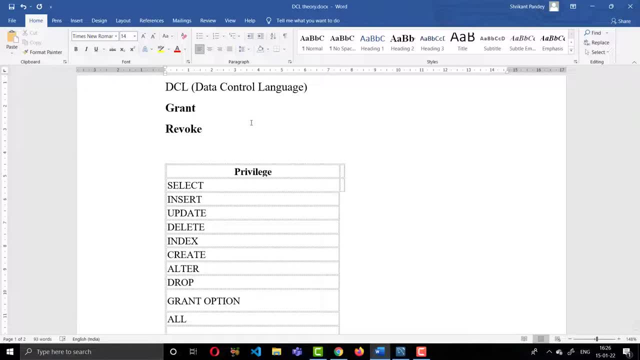 are working on the project, and so you alone you are working on the project. for the some reason you are going somewhere. you are not able to do anything, so you are not able to do some operation on the tables in databases. so now you assign task to the another candidate. 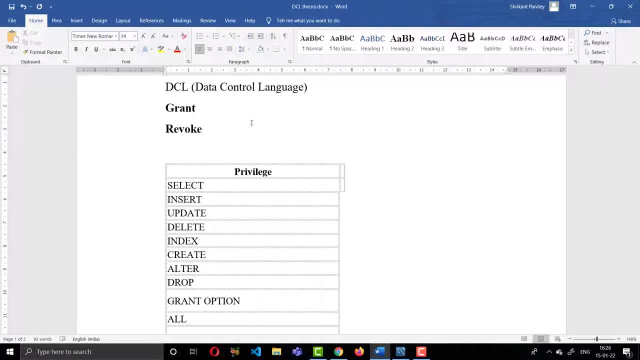 but- and you set the permission for that user- he can only do some limited operation on the tables, like he can only insert the data or he can only select the data. i don't know. such kind of property you can set for the users. so this is the real example. so now you can. 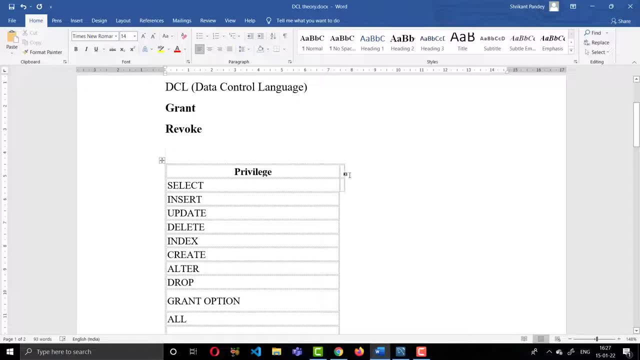 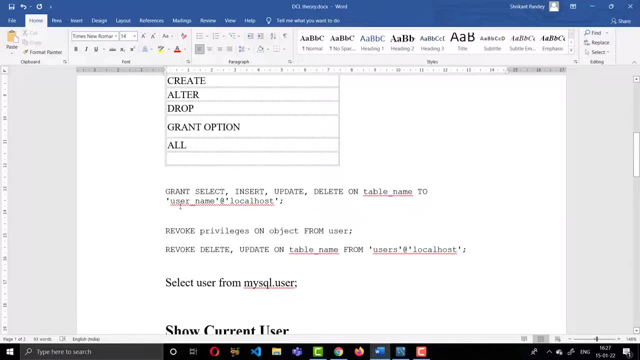 do some operation on the tables in databases. so now you assign task to the another candidate. so this is the real example for the dcl, a data control language in the sql. so uh. so before moving and give the demo of grant and revoke, let's understand how you can show the number. 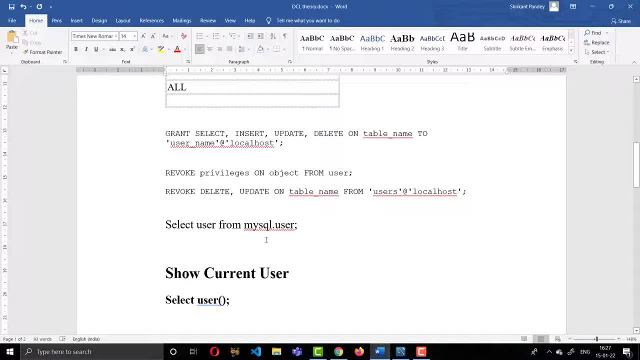 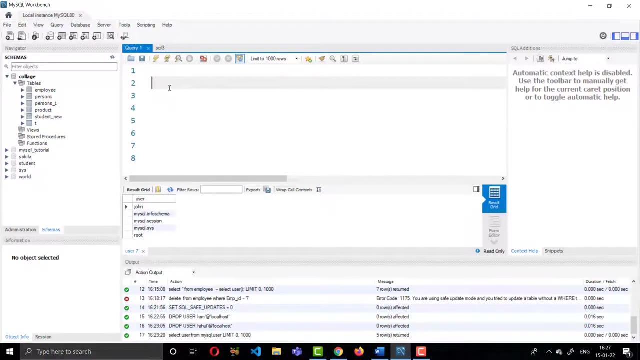 of users in the mysql community server or mysql database. so select user from mysql dot user. so let's copy this part. and i have already opened mysql engagement, so paste here and run. so if you see that user column is appeared. so in the user column here is: uh, john, one user is here: mysql dot input schema. mysql dot. 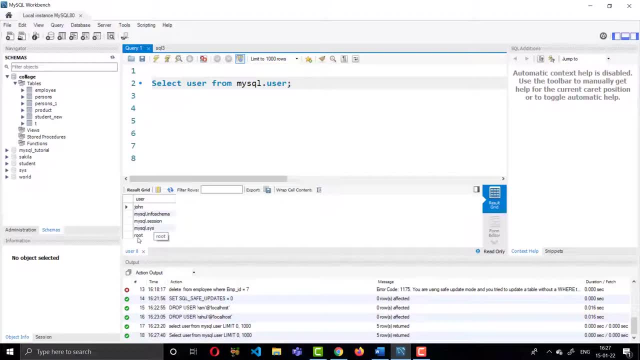 station, mysql dot system and root. so this is the means. uh, default four user is available. i have already added one user, that is the john user. so if you want to see the who, the current user, So type here. let me comment here because later we will require to select user and 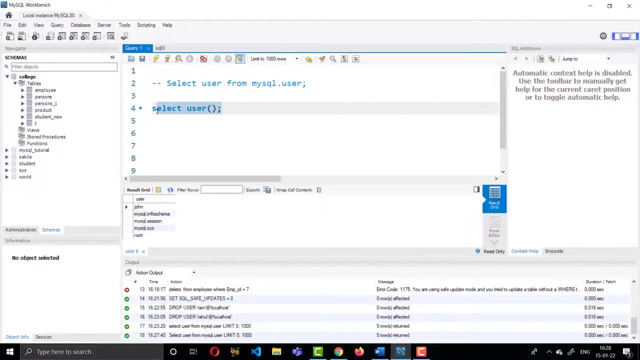 left and right parentheses, semicolon. so this is the. our current user is the root user, so root, our current user is the root user, so he can do any kind of operation. drop the table. drop the data which is. insert the data. delete the data. update the data. 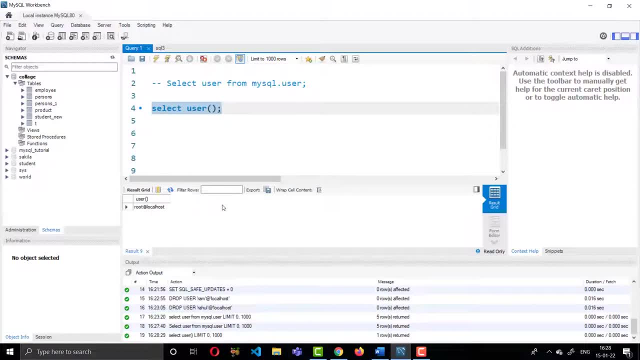 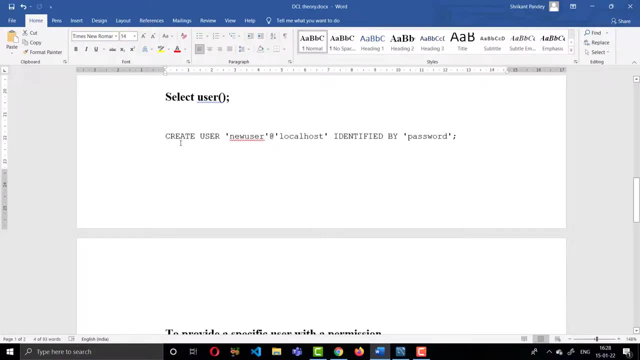 all the privileges root user have. so let's see how to create user in MySQL database. so here syntax, how you can create a data, create user, give the username and at the right localhost, because we have we are doing in the local system, so give the localhost as your IP. 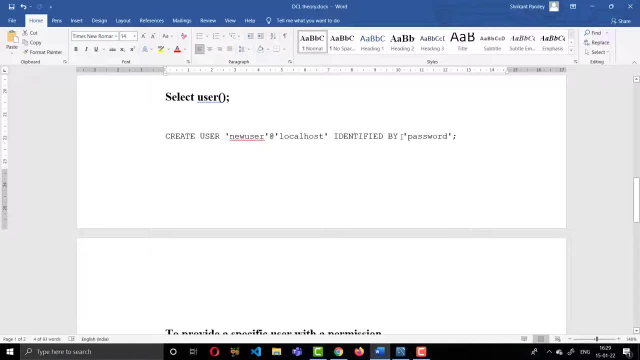 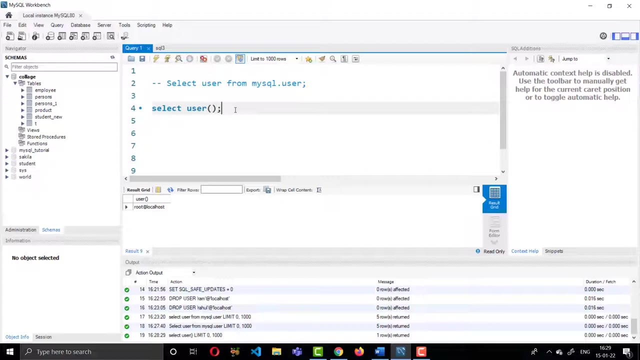 address if you are working on the server. and identify, give the password for the user. so let me copy this here and okay. so create user give, give the username support. I am giving one user ram at the right localhost. identify, set the password for. 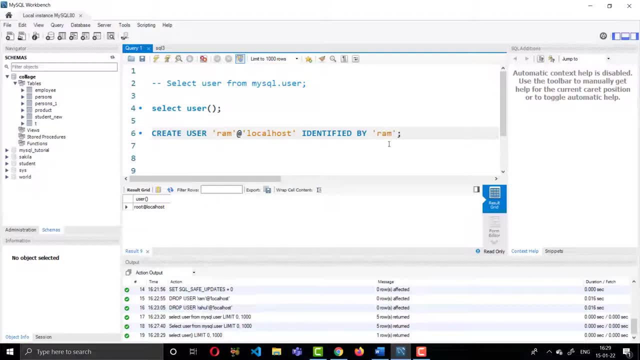 the ram. so I am giving the password ram 1,, 2,, 3, so select this portion and run. okay, so I have already chosen college database. suppose you should run this query. 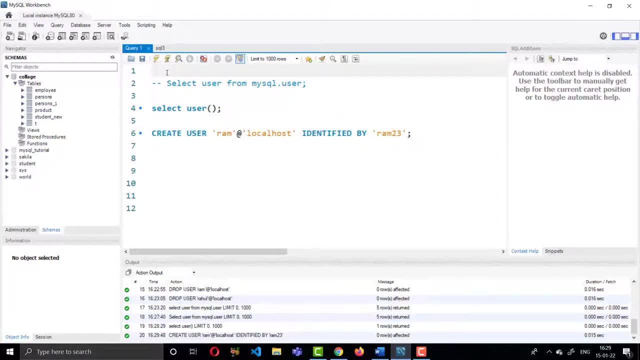 and get error. so you first, you, you select your database. so you would call it and semi-colon as database. so after that you can run this if you get error. so now the ram user has been created. suppose I want to create one more, one more. 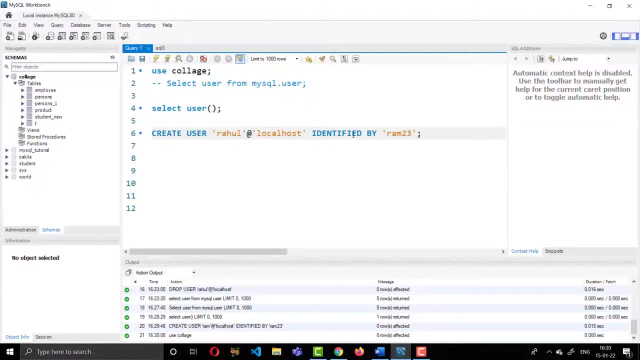 user, ram and localhost. identify and set the password for the ram: ram 1,, 2,, 3, okay, and select this. run here. so the ram user has been created. so let's see, let's verify that the user has been added. 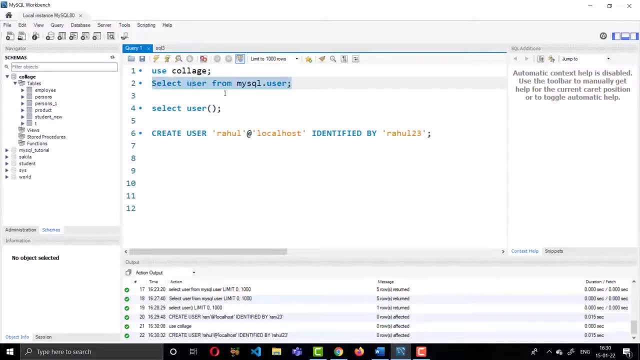 or not. so if you see that select user from mysqluser, so it will list all the user in the mysql. so if you see that ram user has been added, john has already created. so currently- current time- we created two user, ram and ram, so now we learn how to create. 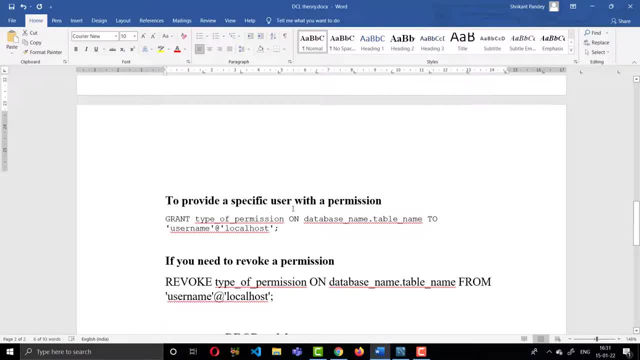 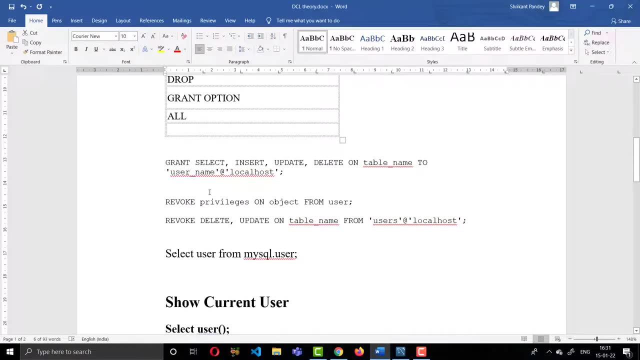 user in the mysql database. okay, okay, so let's see how you use grant and revoke on the table. so for the particular user. so here has a returns of syntax about the grant command to grant, select, so grant. we are giving the privilege here: select, insert, update, delete, you can give. 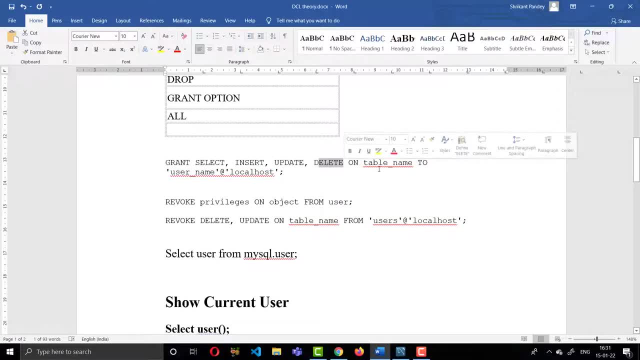 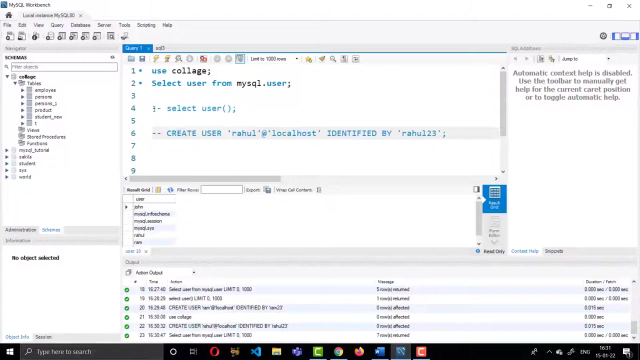 n number of the privilege or the permission for particular table and for particular user. so, table, give the table name to provide your username and, at the rate, localhost. so so suppose now i am commenting this part. so so, so, so, um grant, i am selecting the privilege, select, insert, update, delete. on the employee table. 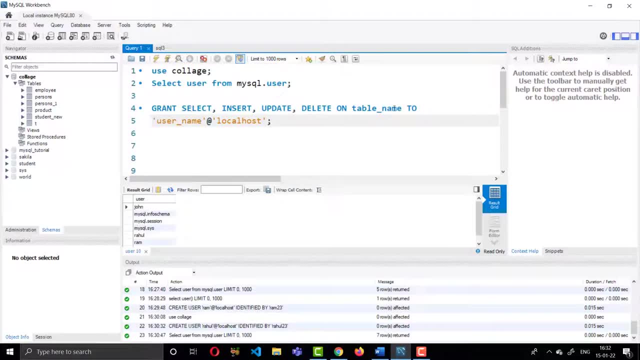 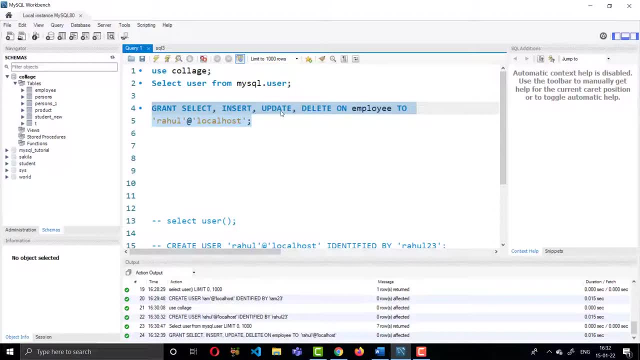 had been shared. so now Rahul will be able to insert, update, delete and select the data formerly employed table. so in the database if you see here person, personal, product, student tables is available. so he not able to perform on the table only he can do operation on the employee table, not other table. so 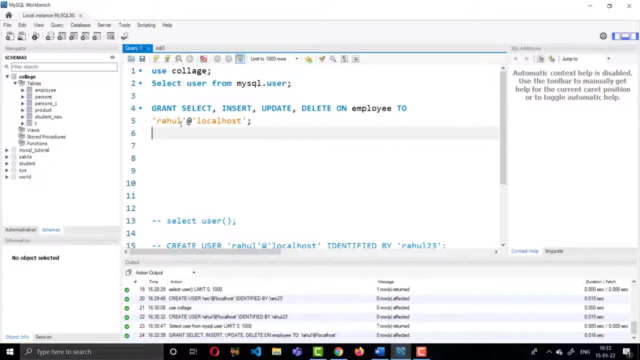 okay, so now we have set the permission for the Rahul. okay, I'm coming commenting here. okay, so suppose I want to insert some data in the employee table by Rahul user. okay, so suppose, insert into my table and give the. you know viewed other columns so I have already. 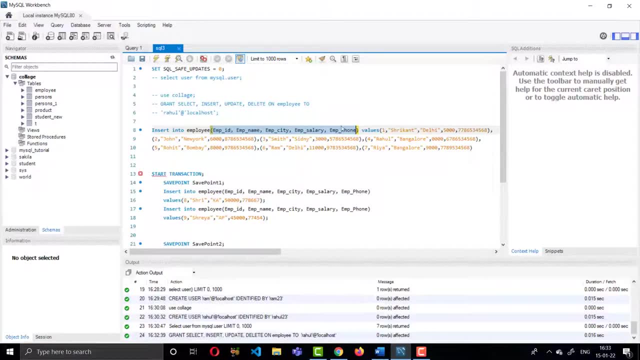 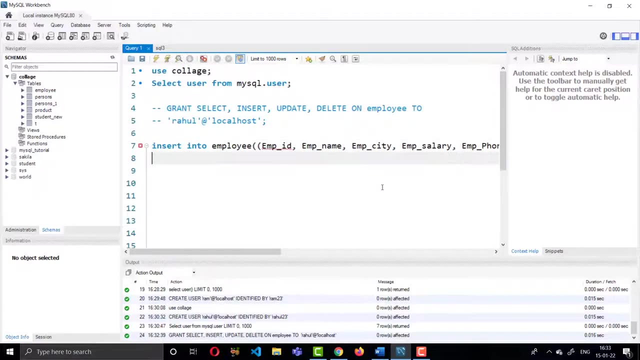 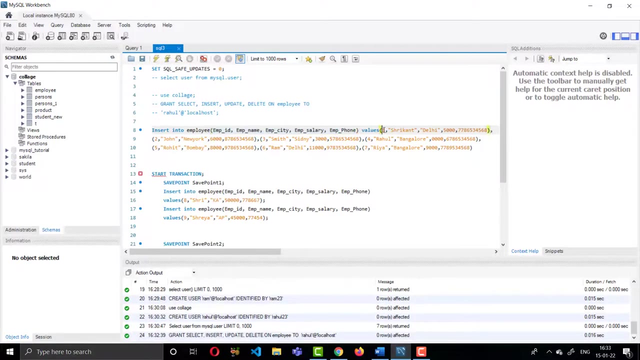 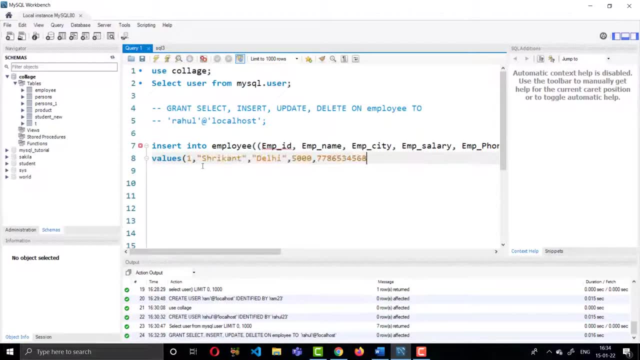 so enter values and I'm inserting only one value. so enter values and I'm inserting only one value. so suppose here I'm giving the ID 10 and here I'm. so suppose here I'm giving the ID 10 and here I'm giving some name, like the chic. 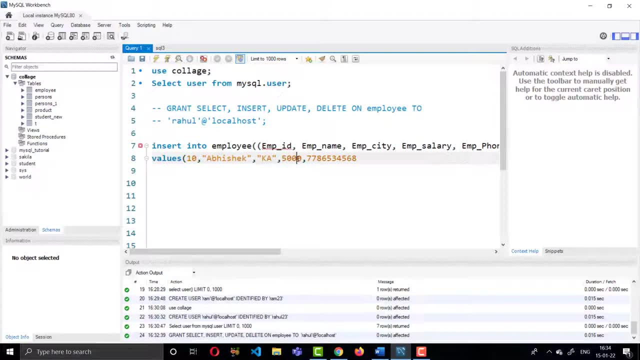 God, God you can say and and give us okay, okay, Insert into employee. give the your column, name and structure of the table and value. in the value, give the values. If you see that data has been inserted by the Rahul user and if you want to see the, 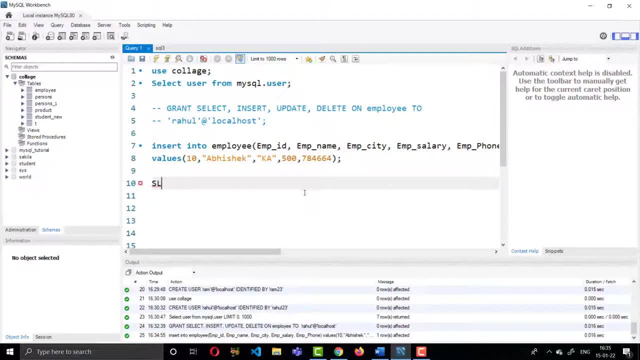 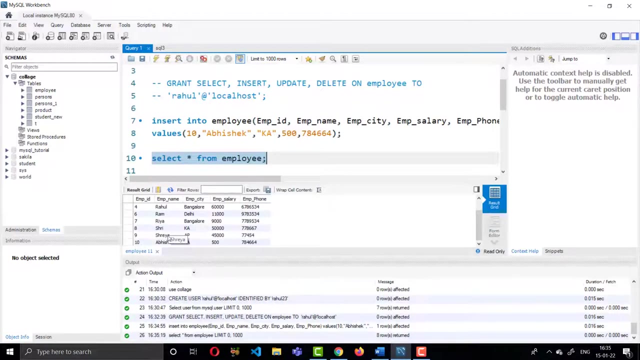 structure of the table select. this information has been added by the Rahul user in the employee table. Okay, suppose you want to delete the data by the Rahul user, So how you will do So. first of all, as you know that the dml command, by default the MySQL database, is enabled. 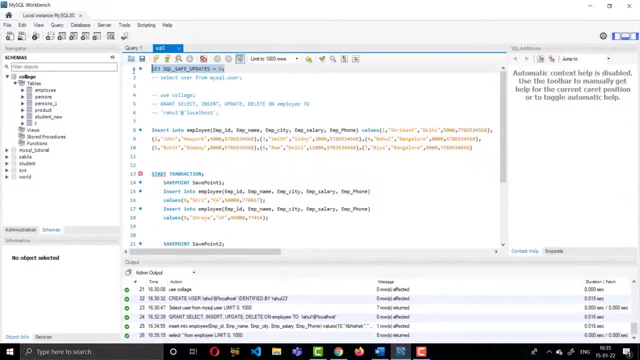 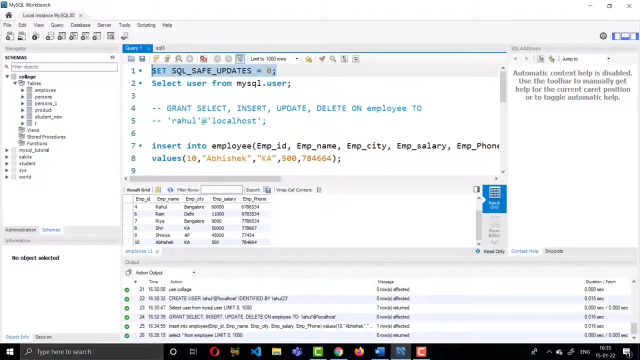 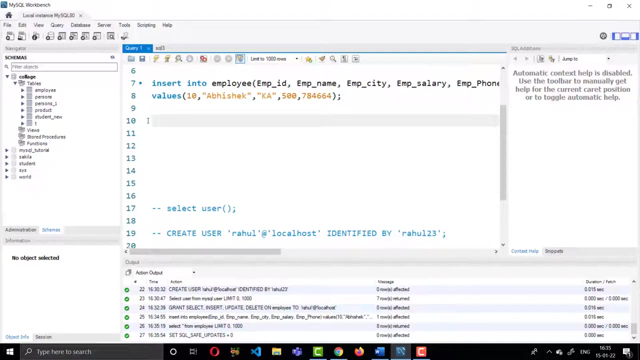 So we have to disable. So for that we will use this command or the query: Okay, Okay, And after that we can delete our data. So delete, delete from provide your table name. so that is the employee and we want to delete. suppose I have inserted this ID number 10 with a shake value. 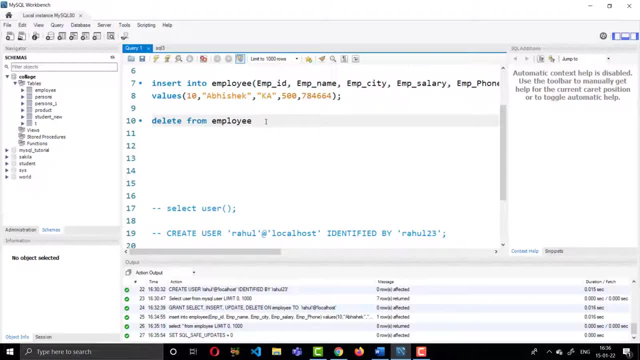 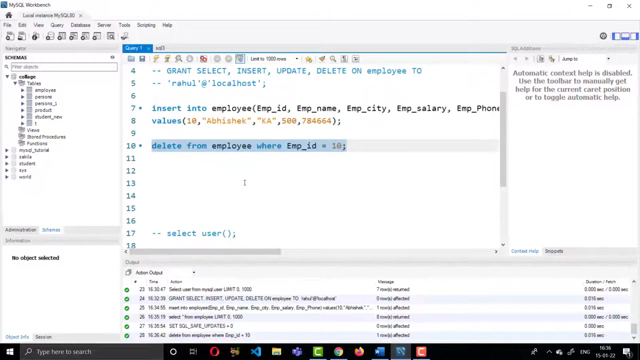 I want to. So delete this ID. So delete from employee where employee is equal to 10.. So let from the source If you see that the information hasn't been deleted from the employee table by a Rahul user. So if you want to see, so let me run again. select this. 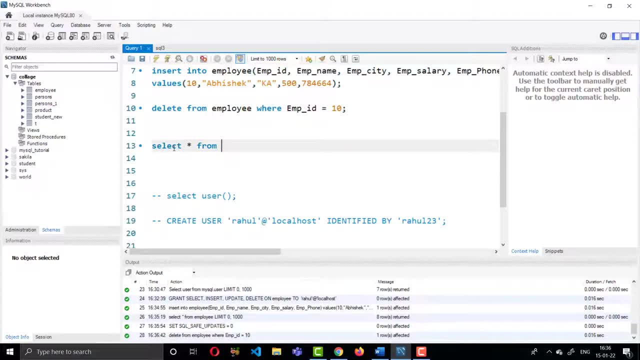 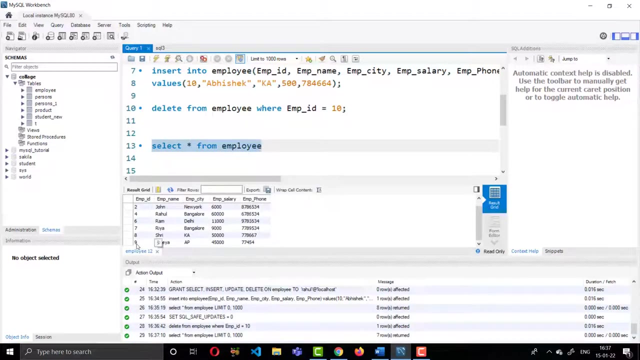 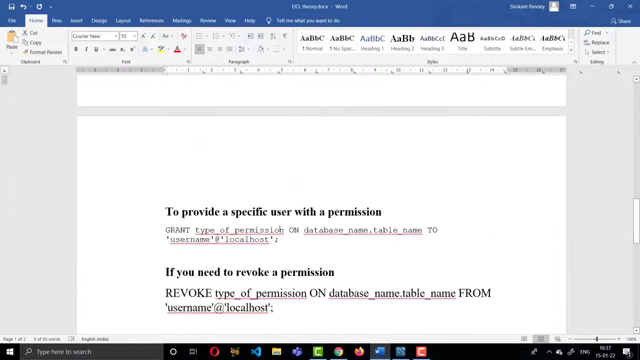 Wow, you see that the ID 10 is not appeared. it means that data has been deleted. so means this is the use of the grant command. so you can select, you can give a number of the privileges or the permission for the particular table, for the particular user. okay, so now let's move. how to revoke the 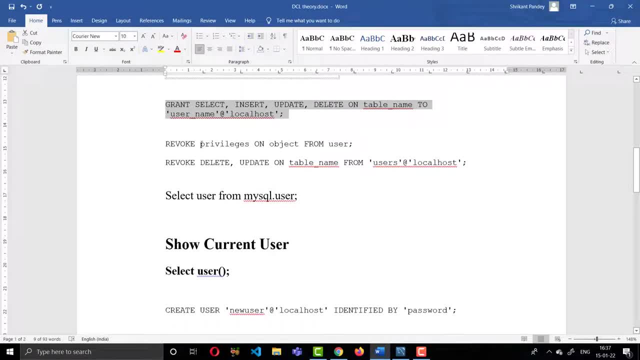 command. so let's understand the command syntax. for the revoke command to revoke privileges. give it the privileges. what kind of permission you have set for the user. give the privileges on object, which means the table name from user. so suppose so initially we have set select, insert, update, delete. 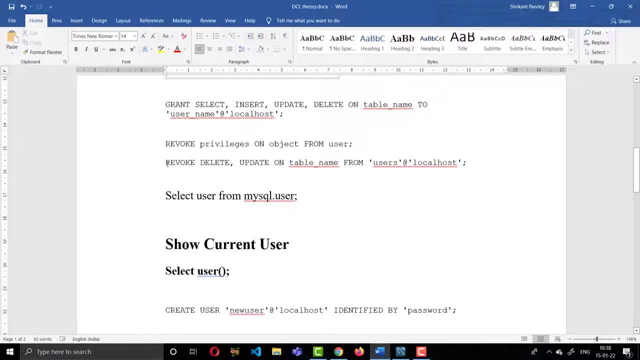 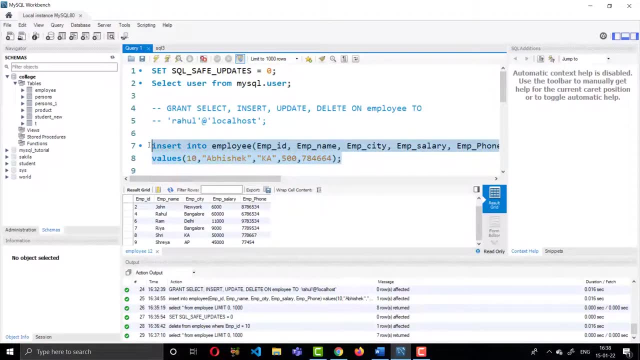 unemployed table by Raul user. so I want to revoke, so revoke, delete. so I have selected select. this also because we have provided select, select, delete, select it insert, update and delete. that doesn't matter. so we are going to, to and give your table name. that is employee and I am. 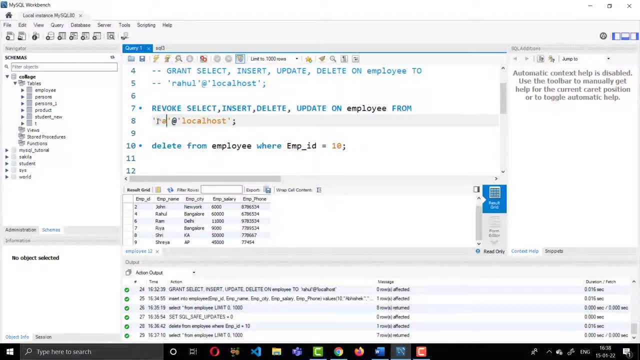 giving for the Raul user Raul localhost. so now I have I want- I am what I am trying to do here. I am taking the changing the permission for the Raul. after that selecting this kind of using revoke command, Raul will not able to select the data or insert the data. delete the data. update the data from the.